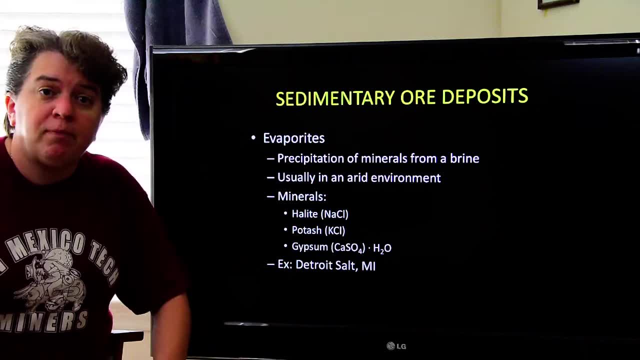 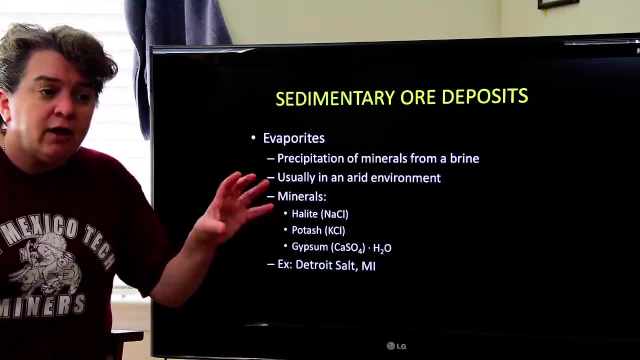 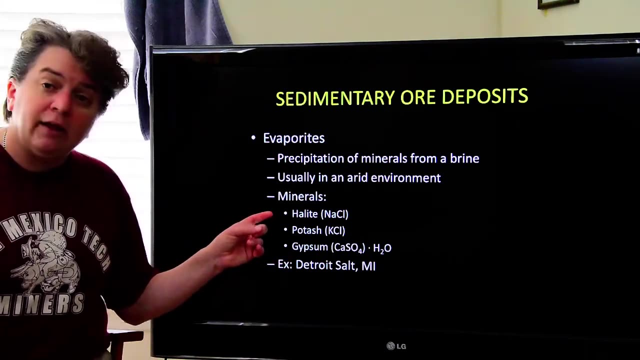 usually going to form in an arid environment, a dry desert type environment, because you're gonna have a lot of evaporation of water there, leaving whatever is dissolved in the water. behind The typical minerals that you get include halite, which is rock salt, right Sodium chloride. That's the stuff we use to 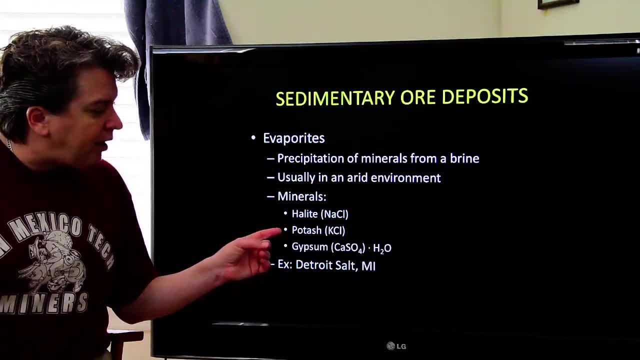 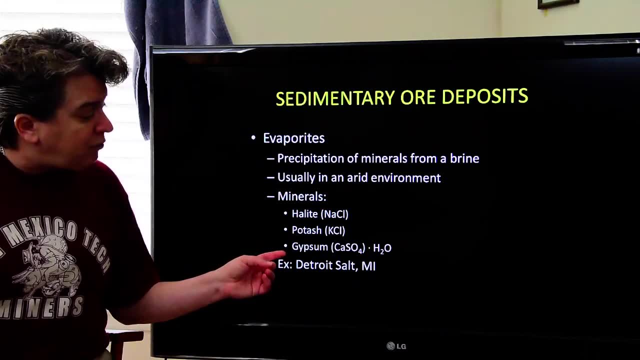 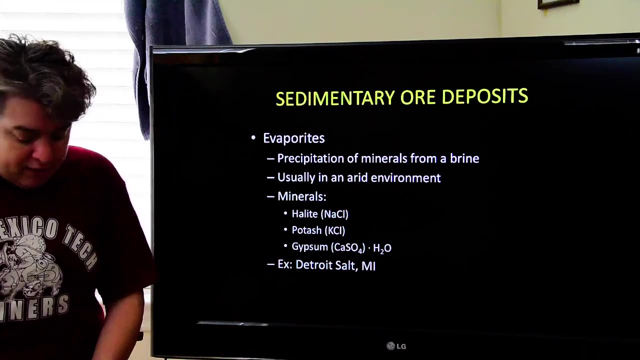 flavor food and do other things with Potash, which is potassium chloride. That's an agricultural mineral. It's used in making fertilizers, Then also gypsum. Gypsum is used in making plaster and drywall, And a great example of a 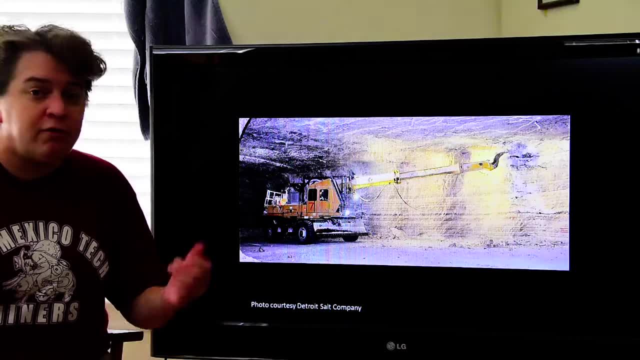 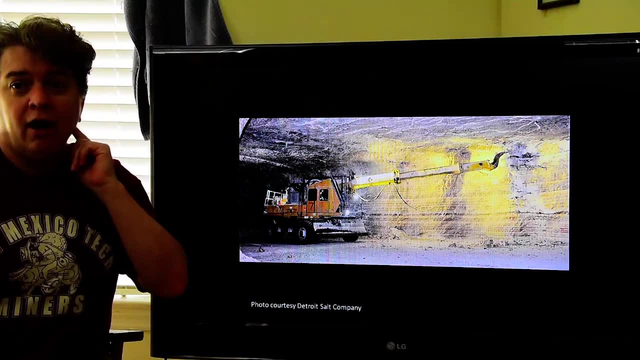 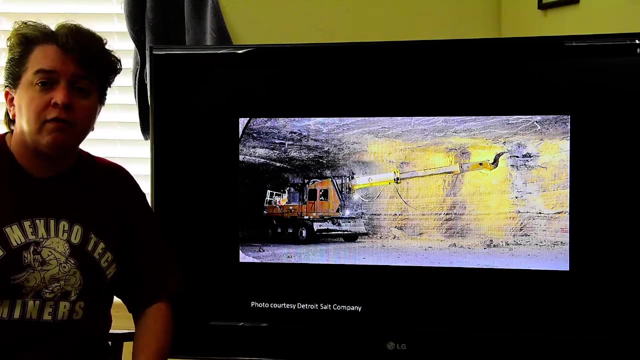 mine that extracts evaporites is Detroit salt And, in fact, if you ever go to the city of Detroit, well, I'm sorry if you have to go there, But if you ever go There, underneath the city is a mine extracting salt that was deposited hundreds of millions of years ago. 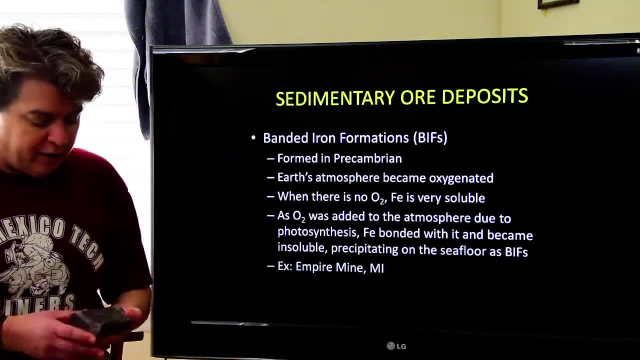 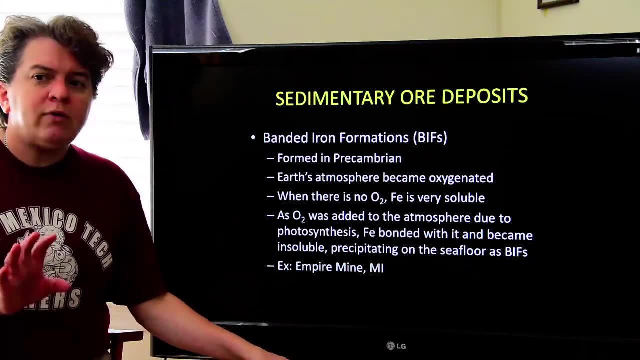 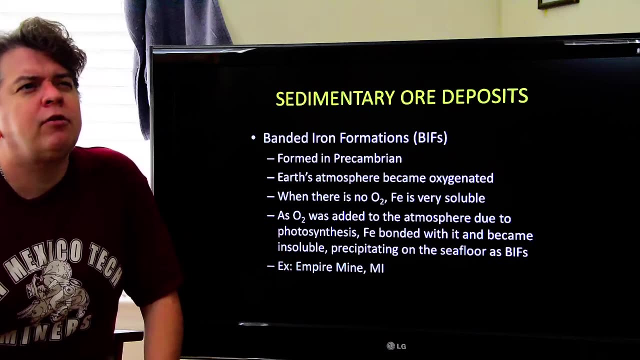 Alright, another sedimentary ore deposit are banded iron formations like my iron ore that I have sitting in your my TV here. These only formed in the Pre-Cambrian, So they only formed really about 1.8 to 2.5 billion years ago. 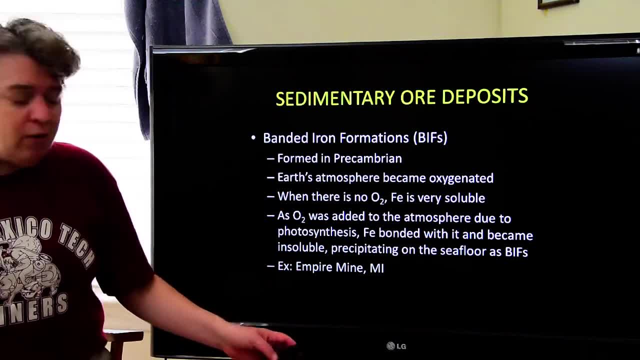 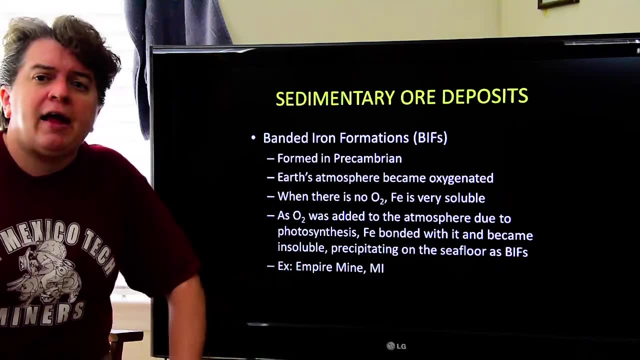 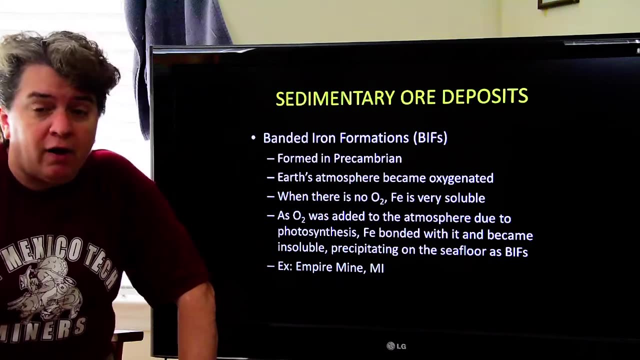 And that's because at that point in time there was something we call the Great Oxidation Event. So early Earth's atmosphere had no O2, no free oxygen in it, And when there's no free oxygen, iron is very soluble in water. 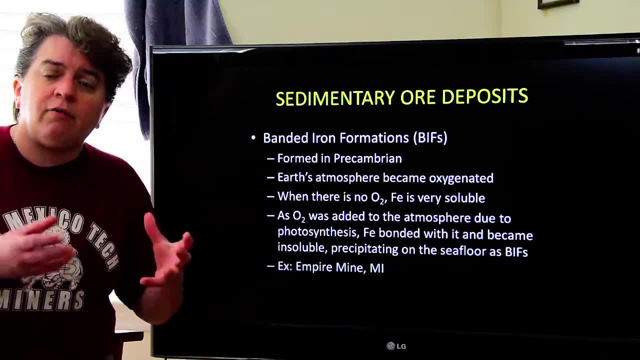 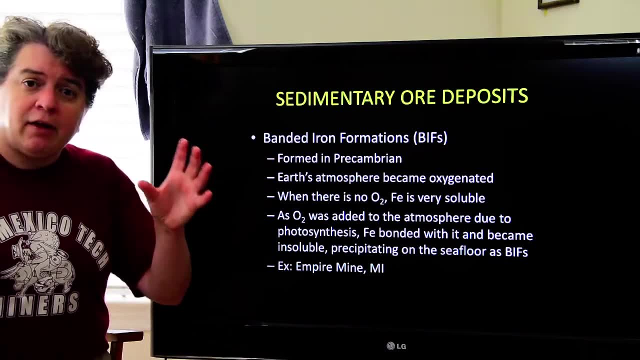 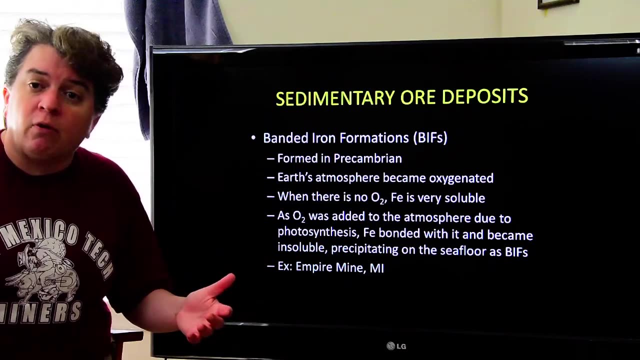 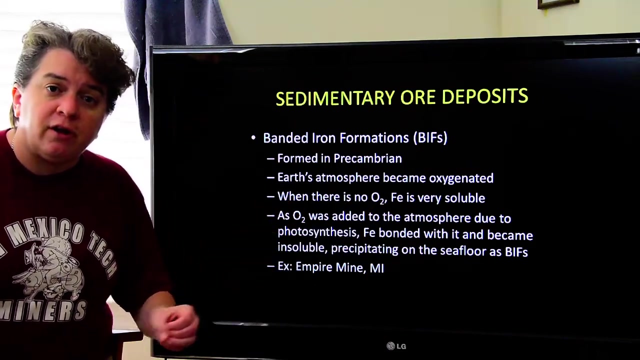 So in the pre-Cambrian time we got a lot of iron dissolved in the world's oceans. But back in that Great Oxidation Event, photosynthesis develops in certain organisms on Earth, And the byproduct of photosynthesis is oxygen. So we start seeing more and more oxygen appearing in the Earth's atmosphere. And when that happens, iron loves to bond to oxygen, And so when there was no oxygen, iron was soluble and it's in the oceans as this oxygen appears. Basically, the iron bonds with it. but when iron bonds with oxygen, it becomes insoluble. 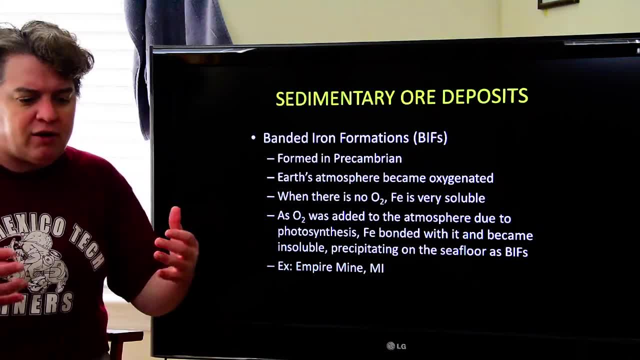 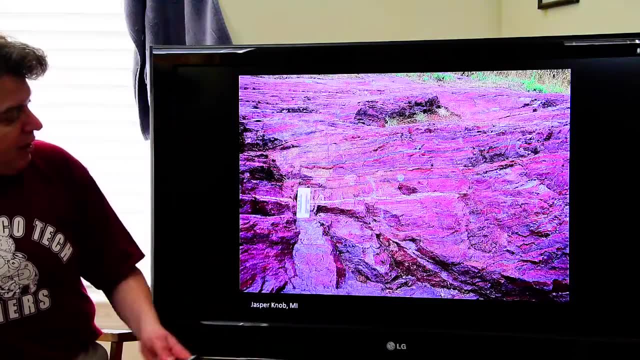 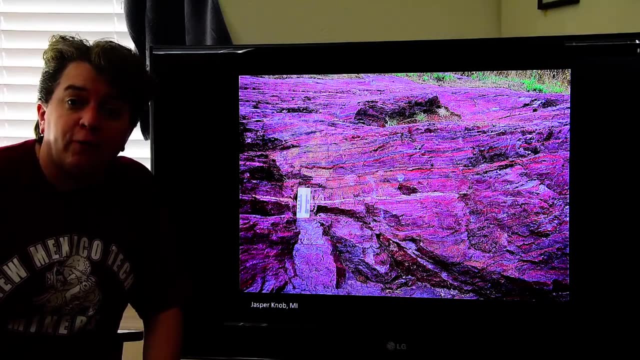 So, as this photosynthesis was producing oxygen, the iron would bond to the oxygen molecules and precipitate to the sea floor And when it did, it created rocks like this very nice banded iron formation we see there, Banded mainly because it has these different layers in it. 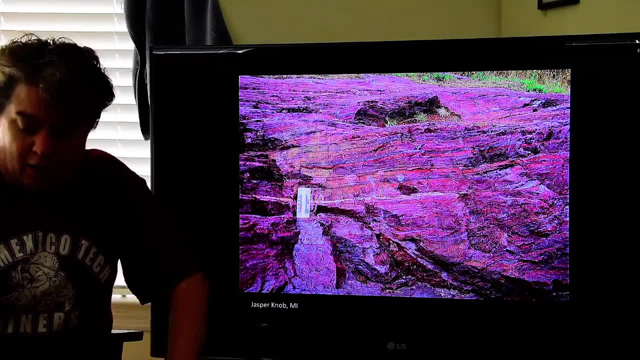 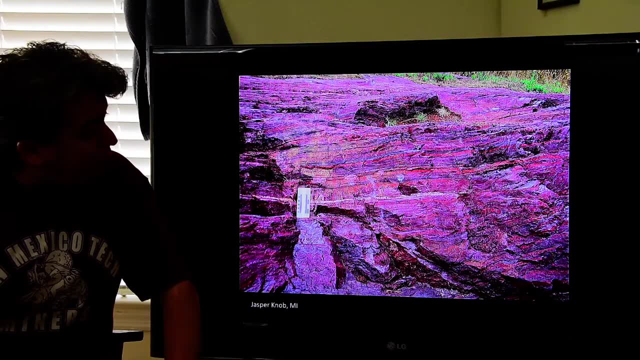 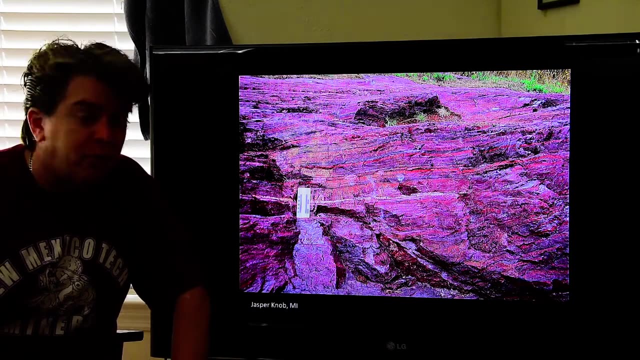 And then, of course, iron formation, because the minerals in there are iron, iron-bearing minerals, iron oxides, And so these are rocks that will never form again on Earth- At least we hope they won't, because if they form again, that means we lost oxygen in the atmosphere. 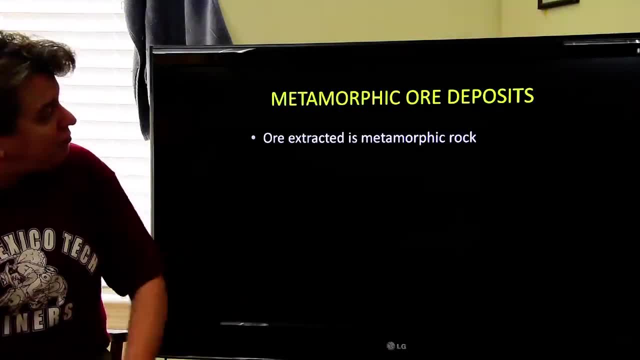 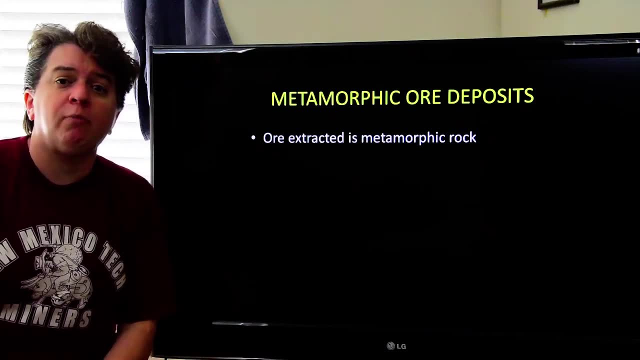 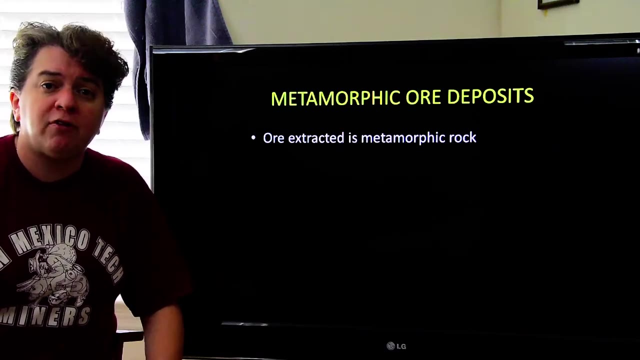 So, anyway, that's banded iron formations. Now there are many other sedimentary ore deposits, but I'm not going to cover those here, So let's move on to metamorphic ore deposits. In this case, the rock that we are extracting from the ground is going to be a metamorphic rock. 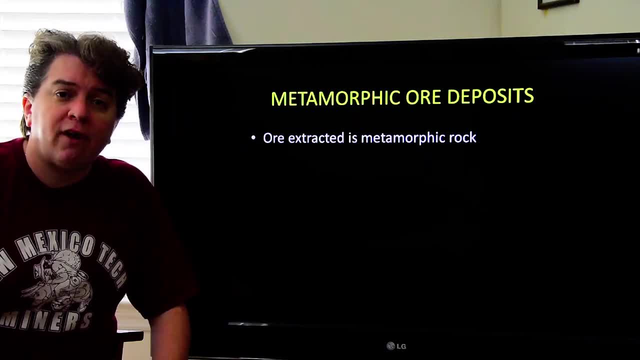 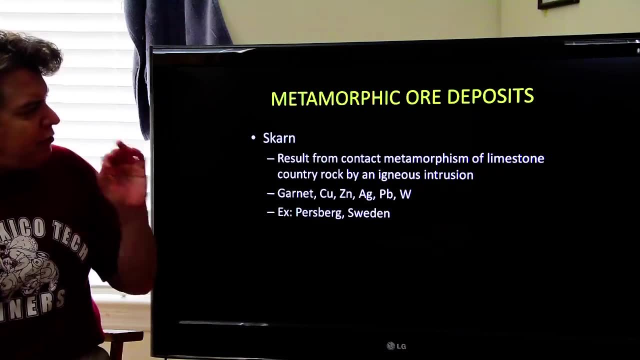 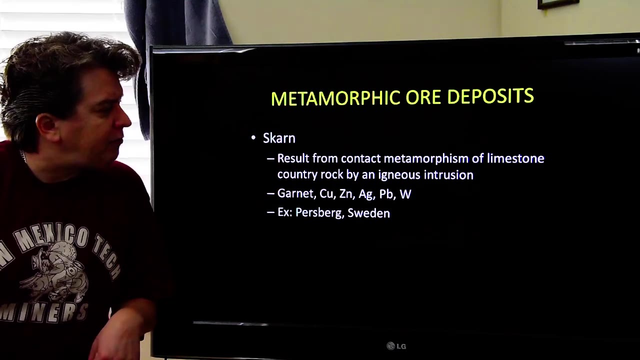 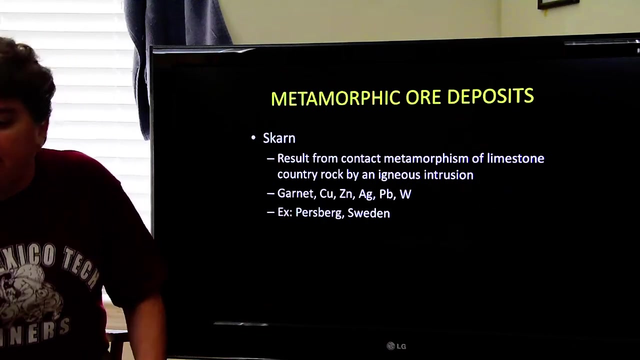 Metamorphic rocks are altered by heat and pressure from their original rock type, And a good example of a metamorphic ore deposit is something called a scarne, And a scarne develops from what we call contact metamorphism, And this is where we have one of those igneous intrusions. 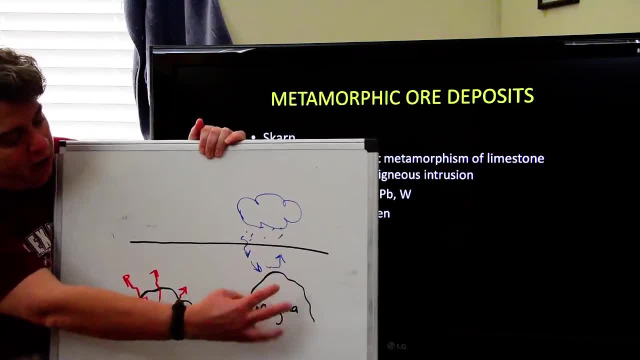 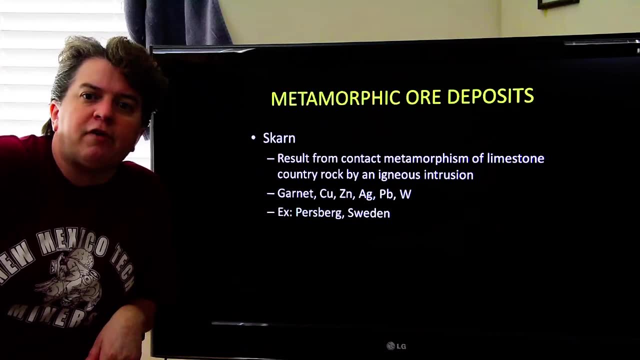 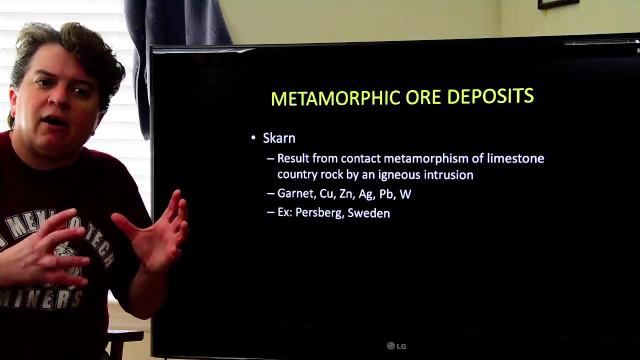 This igneous intrusion is rising through the rock and it's really hot. Remember, those magmas can be over 1200 degrees Celsius. Well, that heat- I just said metamorphism comes from heat. right, The heat of that igneous intrusion is going to end up basically cooking the rock that it touches. 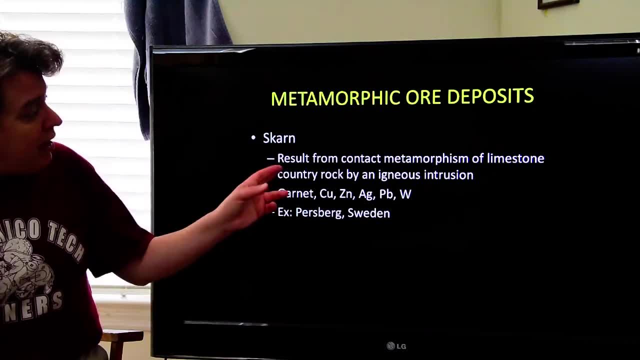 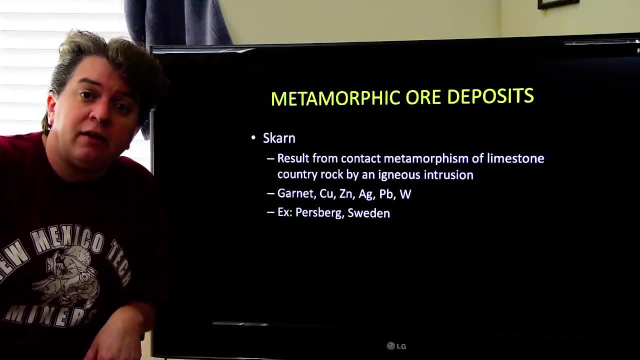 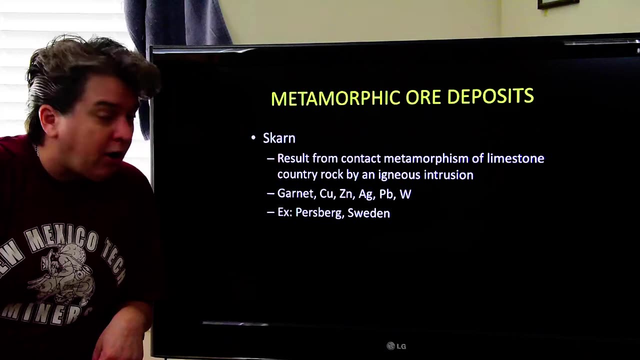 metamorphosing the rock it touches And that's going to be a scarne if that rock is limestone, that the igneous rock is intruding And we get things like garnets forming in scarne, some very beautiful garnets. That's the birthstone of January. 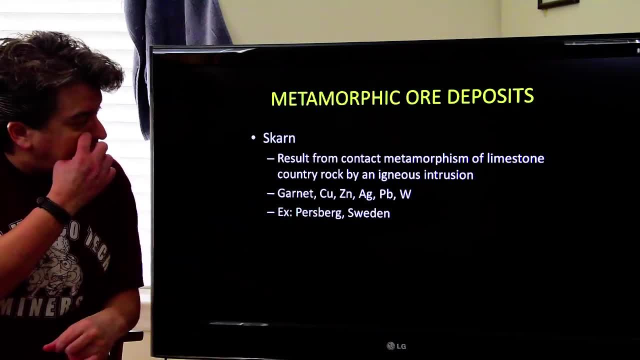 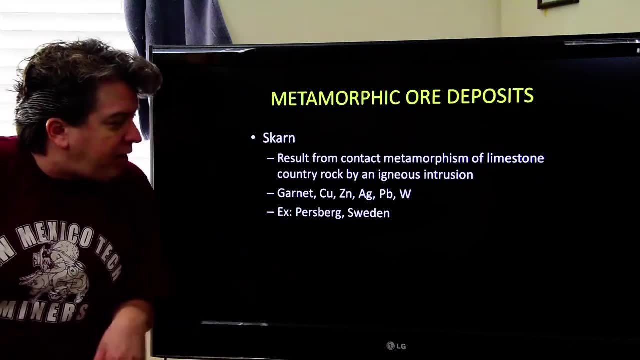 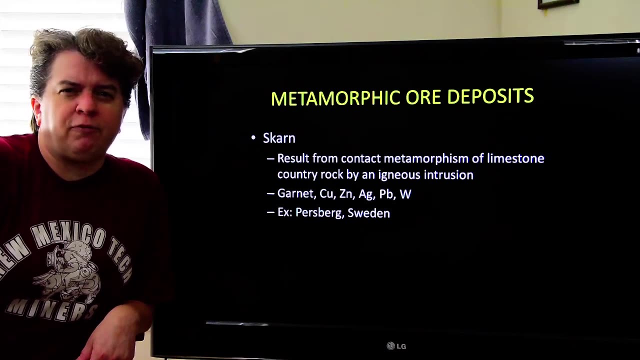 But we also can get deposits of copper and zinc and silver and lead and tungsten, And a great example of one of these is Persberg, Sweden. In fact the term scarne is kind of like a slang term for trash or garbage. 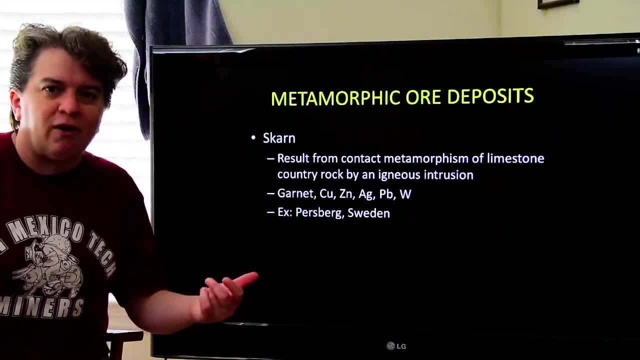 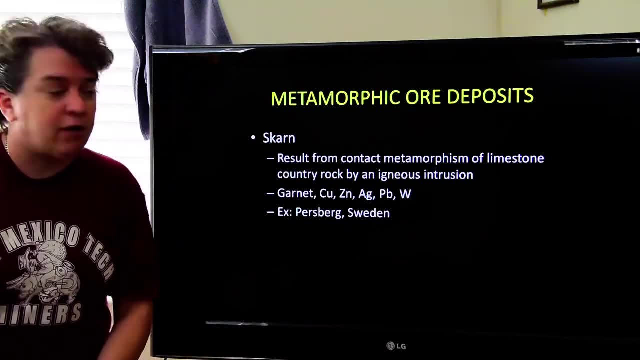 Because originally the miners were like: this is the trash rock, But then they discovered that there is actually a lot of garbage in there And they discovered that there is actually enriched in many of these elements that are actually quite valuable. So that's what we're seeing here. 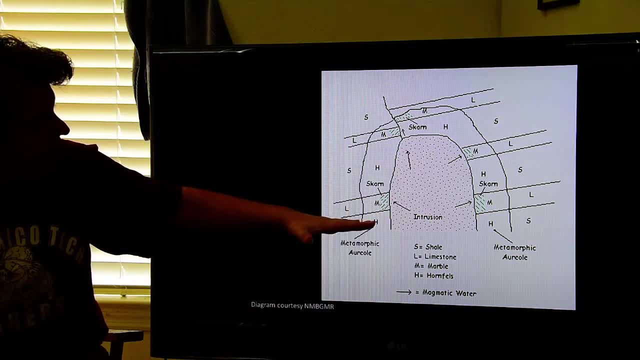 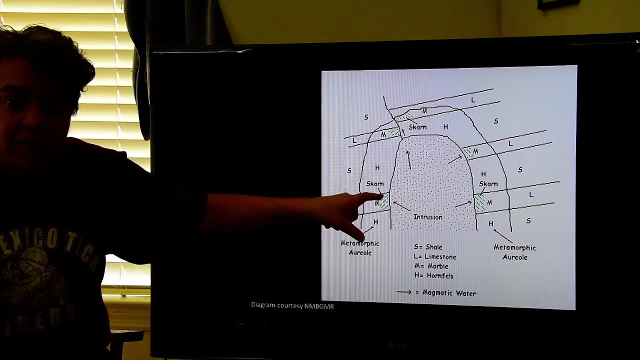 This is my igneous intrusion. And then I have these layers of limestone and shale- limestone and shale- And where the igneous intrusion touched the limestone, it gets turned into a rock type called marble And we have this scarne deposit developing right in there. 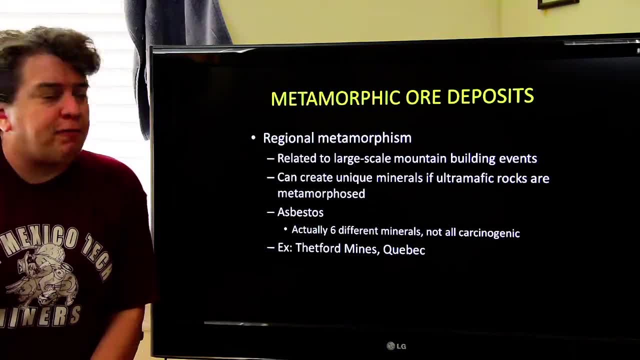 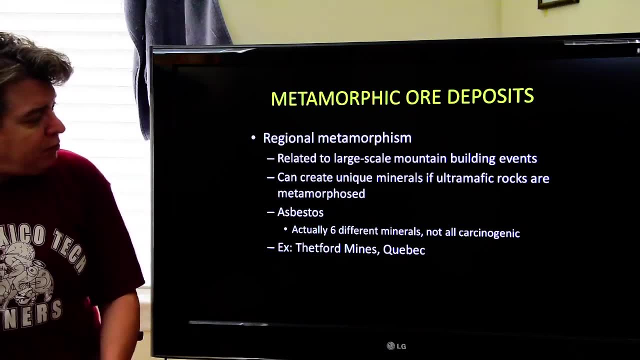 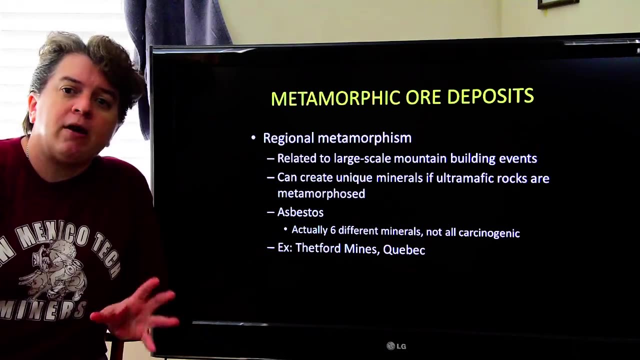 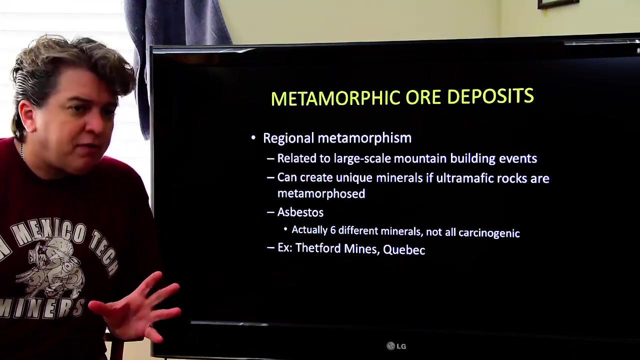 All right. Another thing we get from metamorphism is we get asbestos minerals formed And this forms if you get ultramathic igneous rocks metamorphosed. So ultramathic igneous rocks are things like peridotite And asbestos. it's actually a group of minerals. 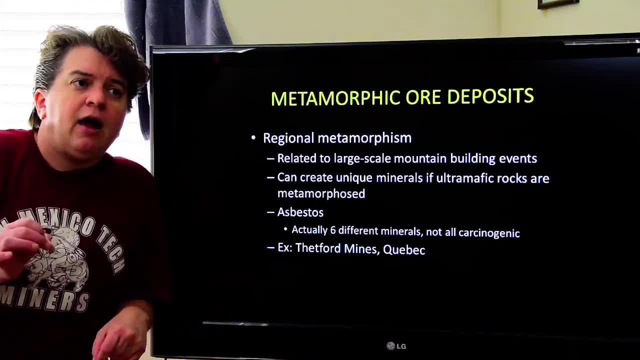 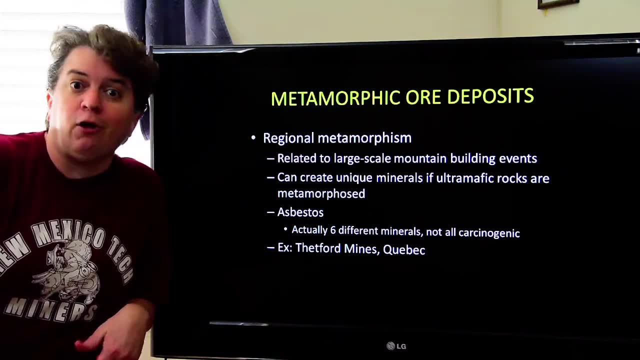 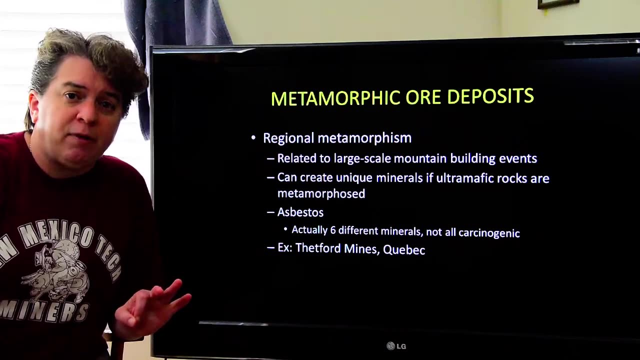 It's actually six different minerals, And what they have in common is they're all fibrous, They're hairy. You can actually weave them into clothing and stuff if you wanted to. And one thing to remember about asbestos is not all. asbestos is carcinogenic. 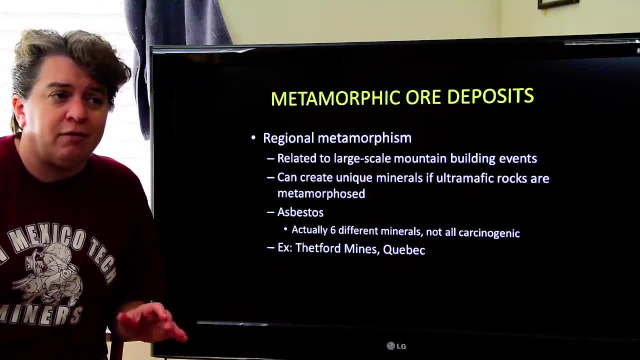 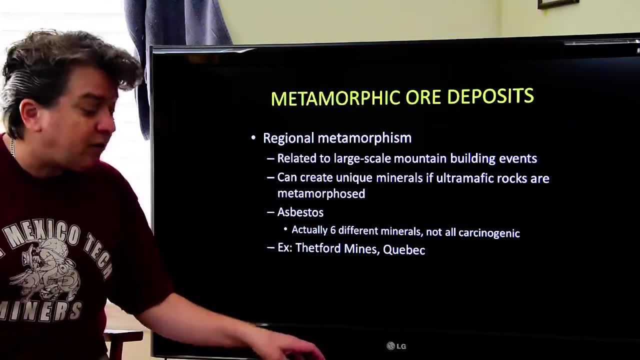 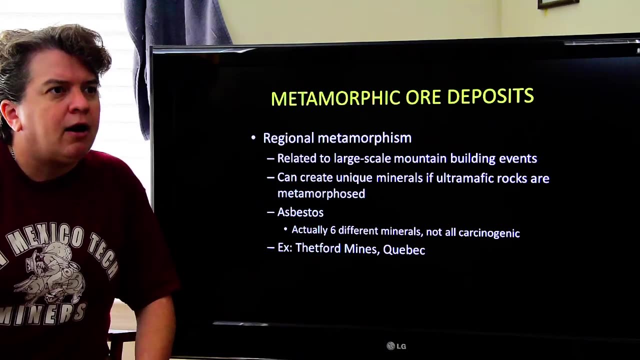 Now I'm not saying: go and sniff all your minerals, because honestly, inhaling any kind of particulate matter is bad for you, But I did want to point out not every asbestos mineral out there is carcinogenic And in your textbook there's actually a little discussion of that. 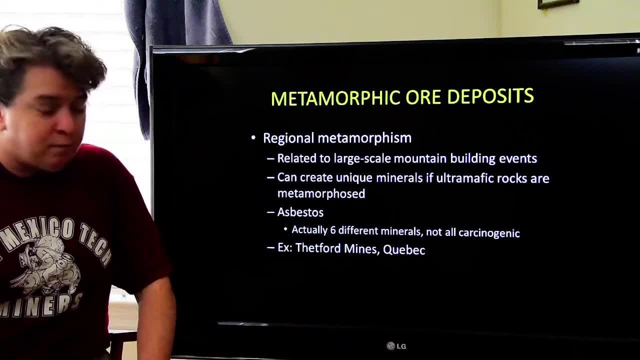 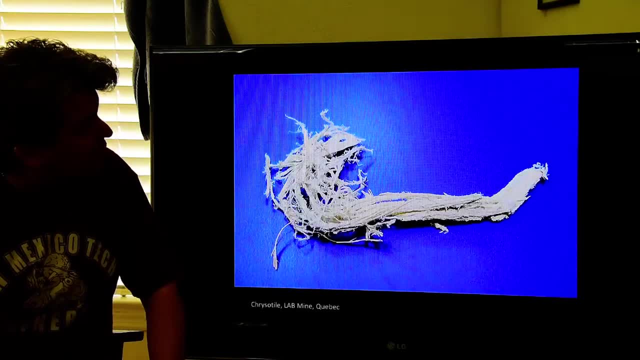 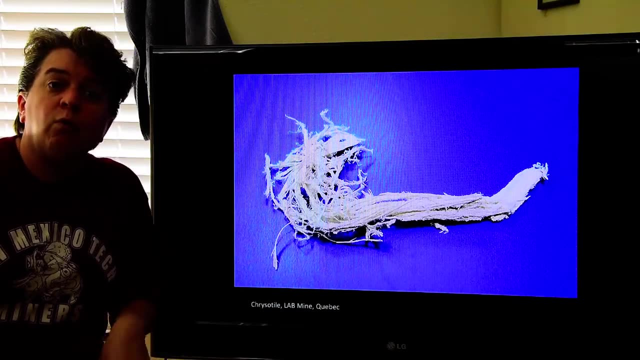 A nice example of a mine that extracts asbestos is at Thetford Mines in Quebec, where this is a mine where they extract asbestos, And that's what asbestos looks like Like. I said it is fibrous And so it can be woven into like fireproof clothing and things. 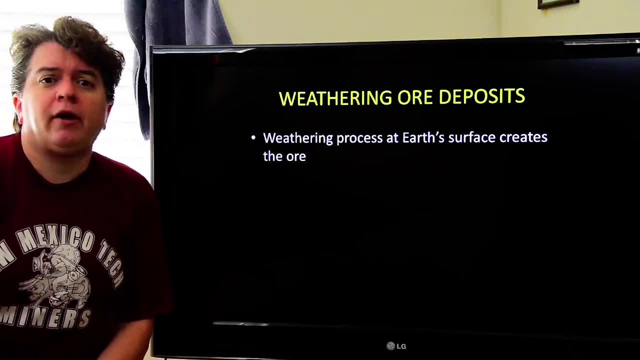 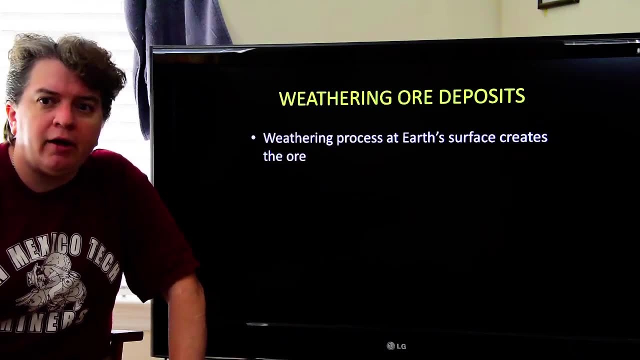 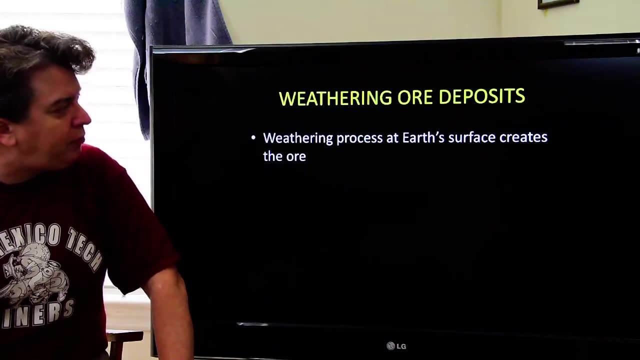 All right, Let's talk about weathering ore deposits. When rocks sit on Earth's surface and are exposed to rain and sun and water and stuff, they're going to weather And we can get a few ore deposits created by these surficial weathering processes. 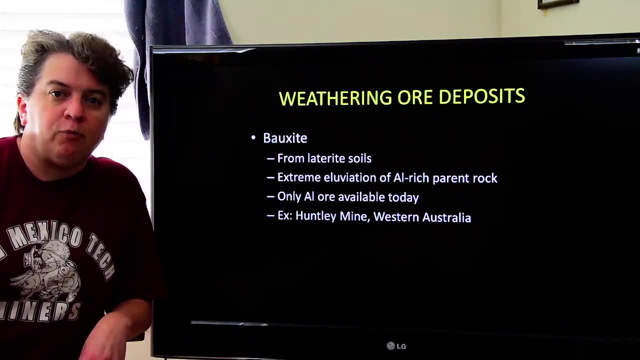 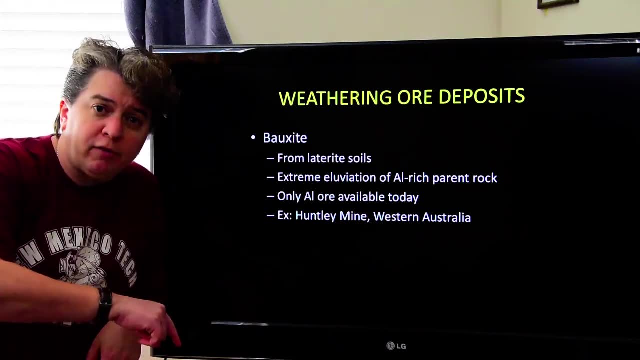 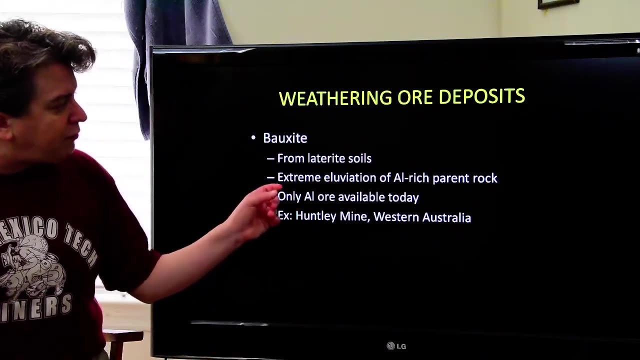 In fact the mineral bauxite comes from weathering. Now bauxite forms in laterite soils And remember from the soils lecture I said laterites are those tropical soils And you get this absolutely extreme eluviation and leaching of an aluminum-rich parent rock. 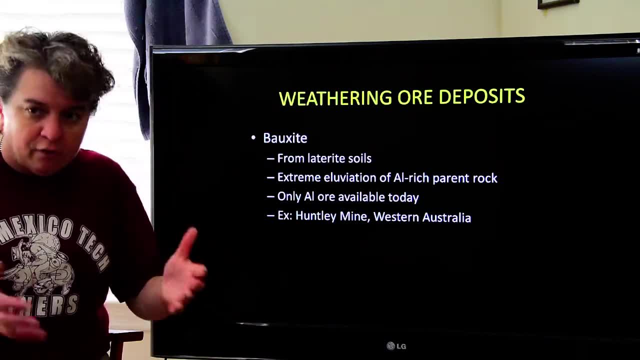 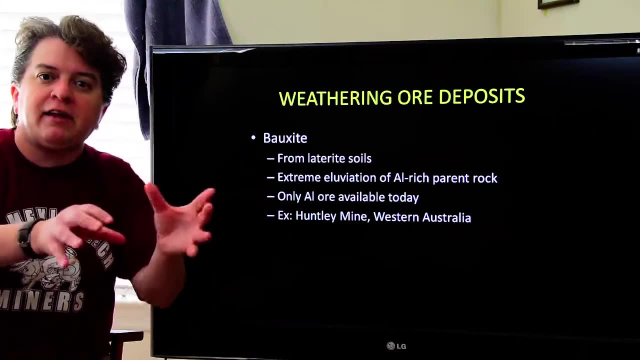 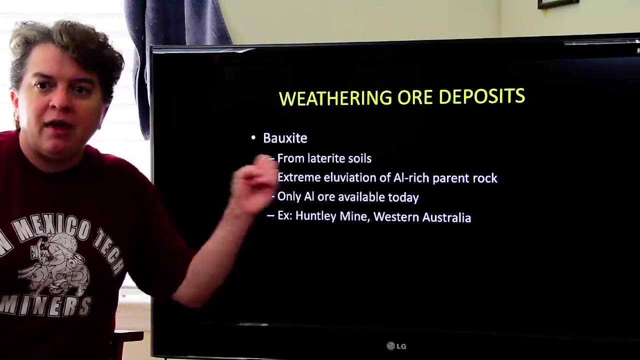 And so what happens in this tropical environment? you have so much rain and so much water going through the soil. it basically dissolves everything that's even slightly removed from the soil, Everything that's even slightly remotely soluble. But one thing that is not soluble at all is aluminum. 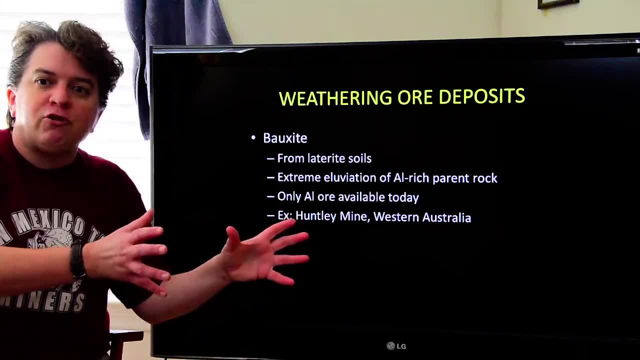 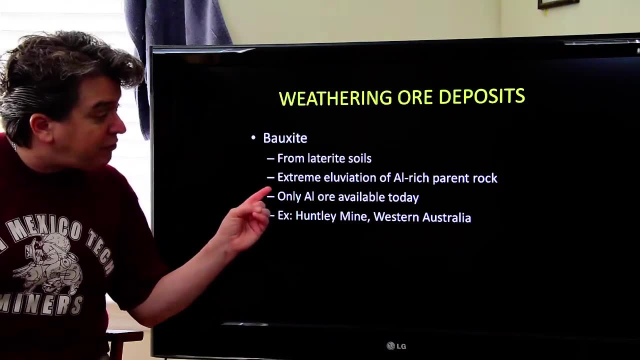 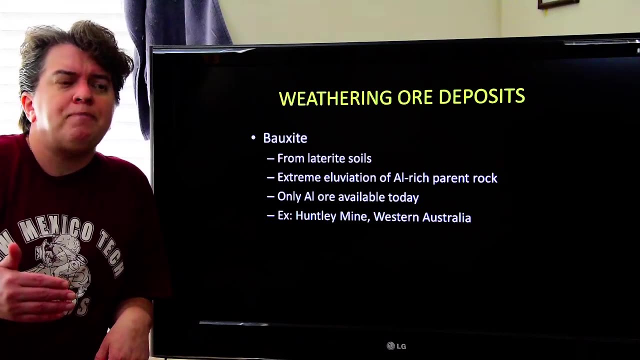 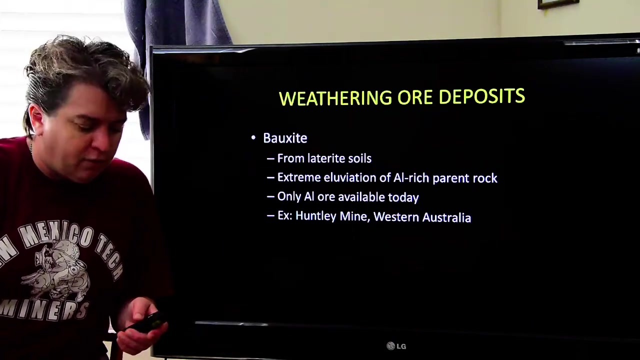 And so everything else basically gets washed away and the aluminum gets left behind, And so bauxite from these tropical soils is the only aluminum ore we know how to process today, Or at least we know how to economically process today. Now, a good mine example is often Western Australia. 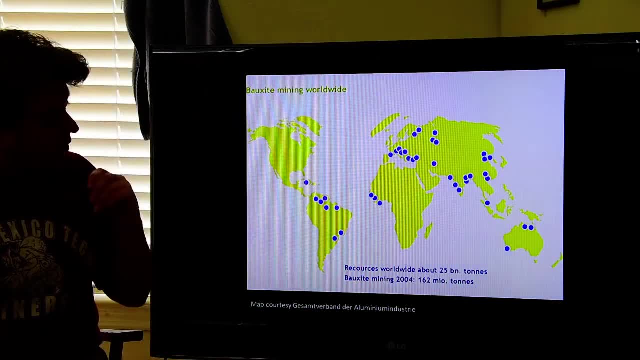 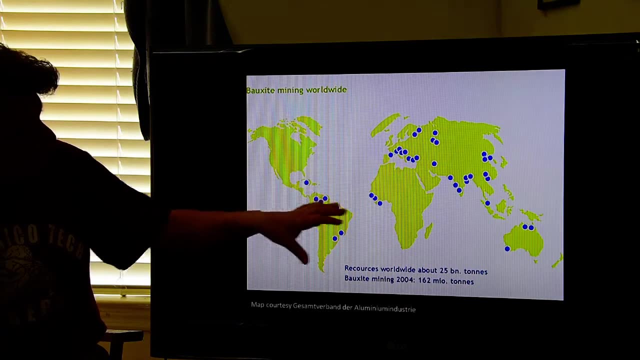 But, as you can see in this diagram, this is bauxite mining worldwide. Now some of them make sense. right, We're in the tropics, we're in the tropics, But then it's like what the hell is going on in Russia. 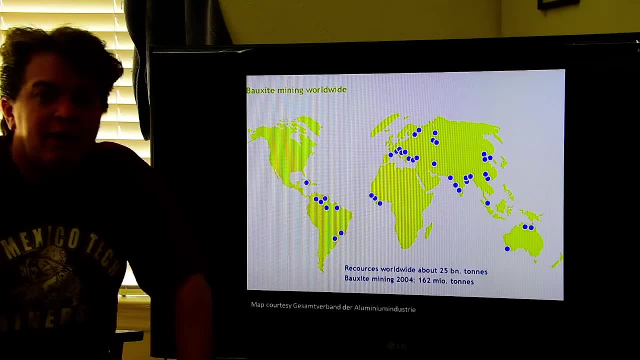 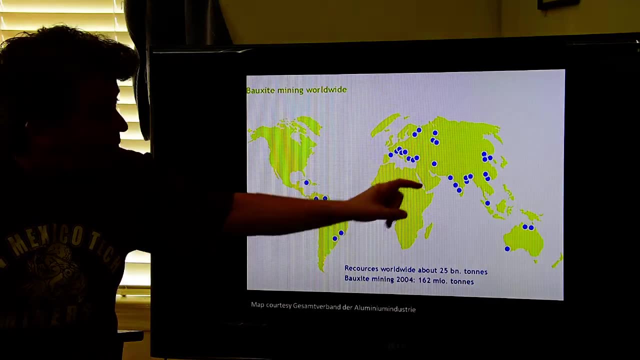 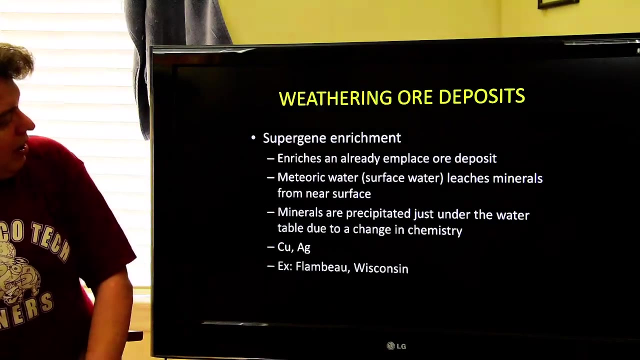 Russia's, not the tropics, And you have to remember plate tectonics right, Once upon a time that was sitting more in the tropics. So those are just some very ancient bauxite deposits. Alright, let's see. 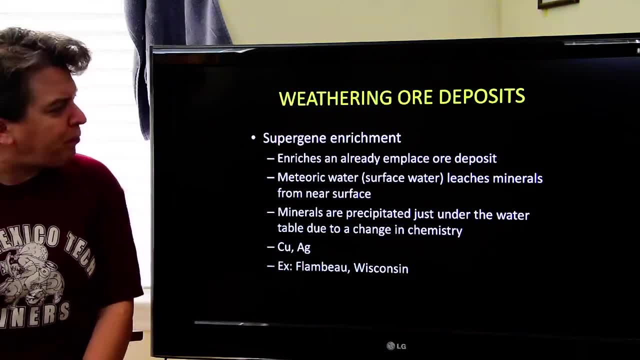 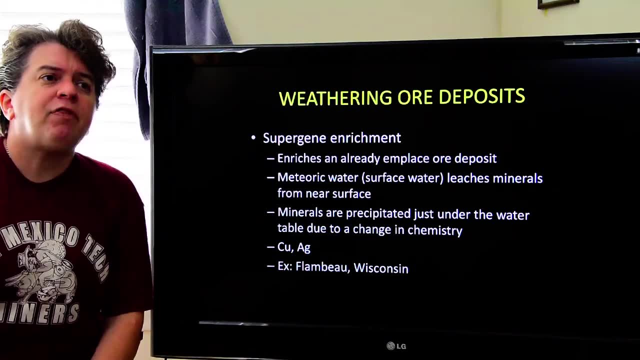 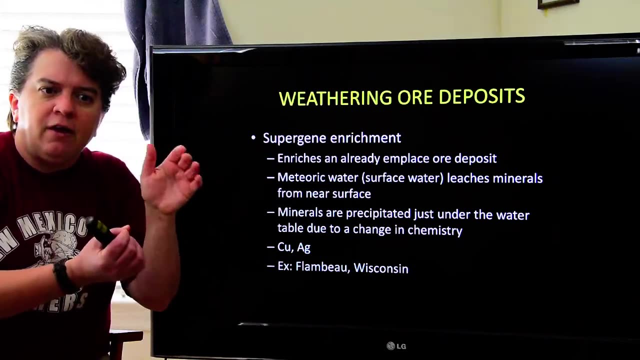 Last but not least, let's take a look at something called supergene enrichment. Now, this doesn't actually create an ore deposit type, But the weathering concentrates and really focuses all of the wealth, all of the economic minerals in a specific area. 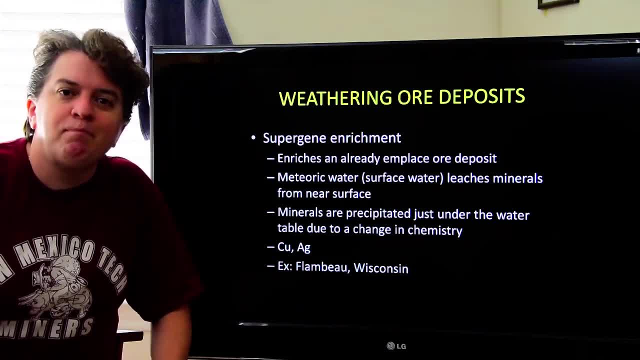 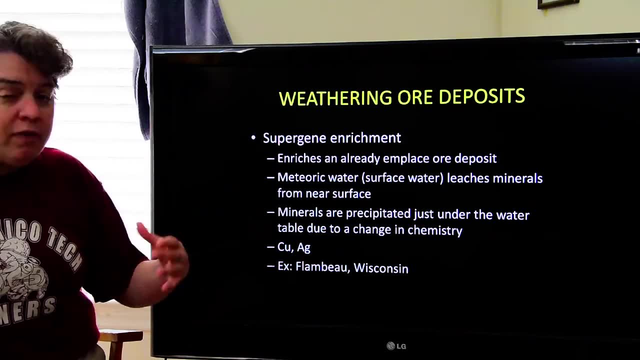 So it really kind of makes an ore deposit better. And in this case we have meteoric water, And anytime you see this term, meteoric water, that just means surface water, And so it rains and stuff and the water seeps into the ground. 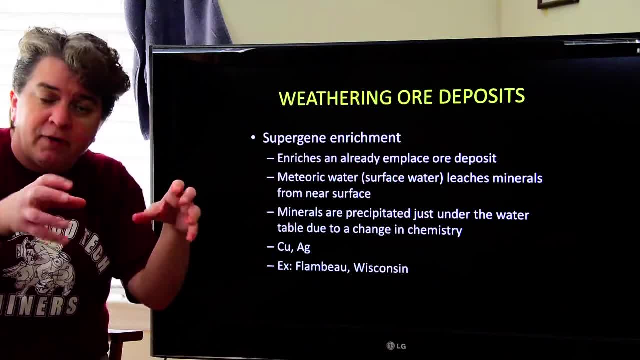 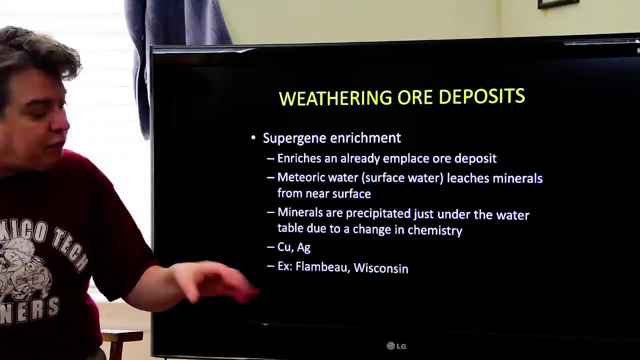 And it's going to leach some of the minerals from close to the surface. Leaching again dissolves some of those minerals And then those minerals get carried downward And because of chemistry changes they are precipitated just under the water table. 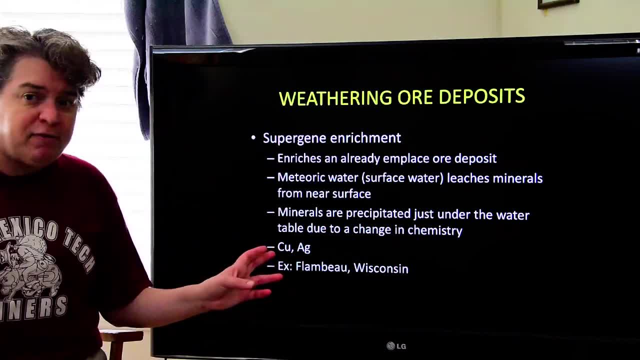 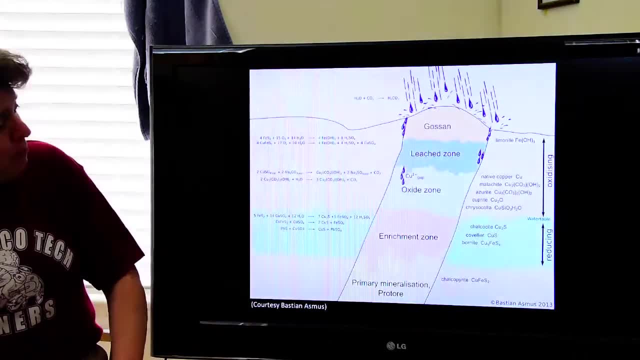 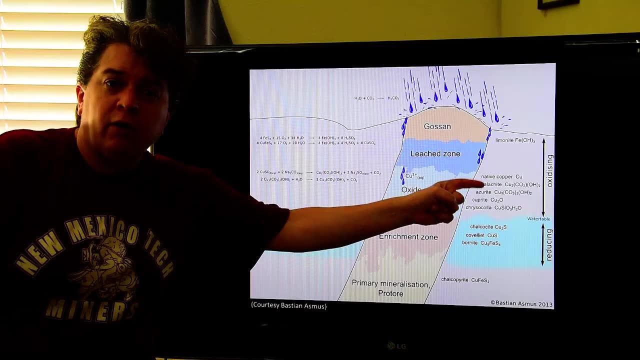 And frequently what you might get in these types of supergene enrichment you can get copper and silver are very common ones. A good example is flambeau in Wisconsin. So what we have here. of course, on the test, you're going to have to know every one of these chemical formulas. 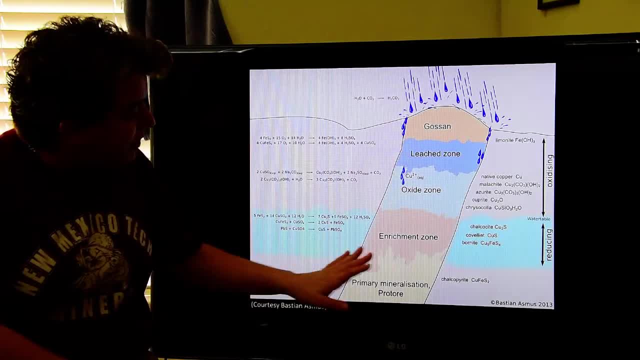 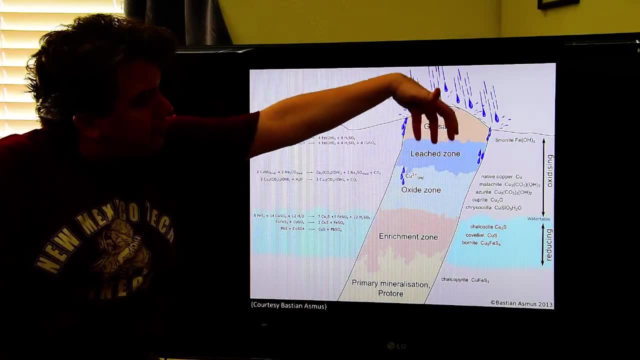 No, you're not really going to have to know that. So let's look at what you are going to have to know Right here. this is my ore deposit And it rains there and it starts leaching. It starts taking away some of the important elements here. 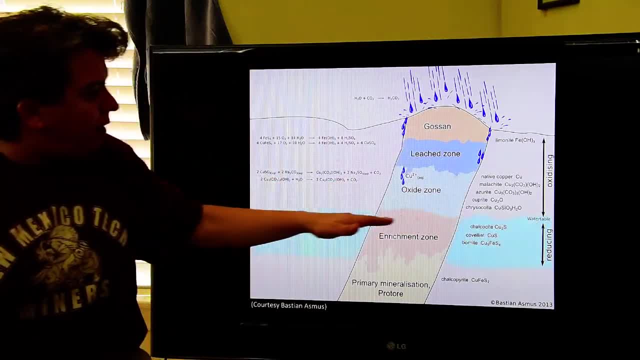 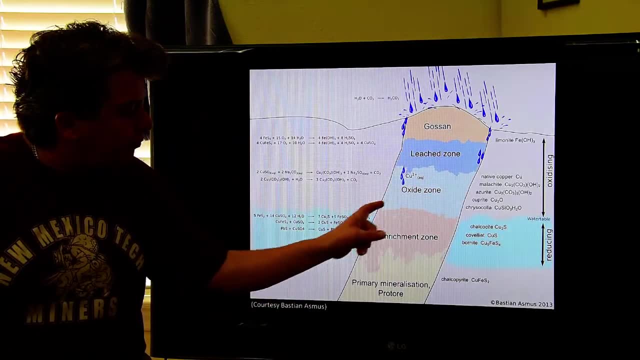 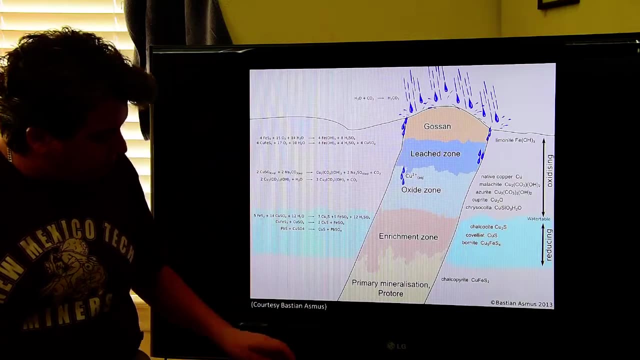 And carrying them downwards. here's our water table And there's the enriched zone. It deposited all of those minerals right down there. So what that does is this is really really rich ore. It really concentrated all the good stuff right there. 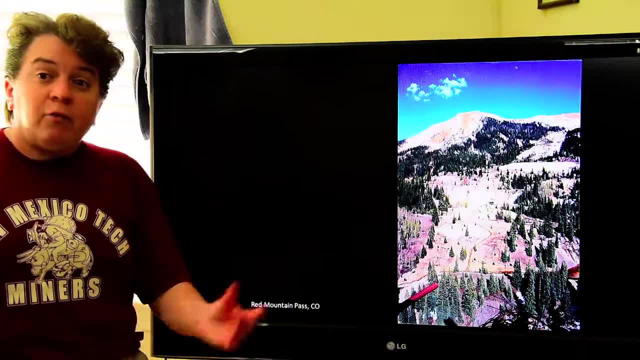 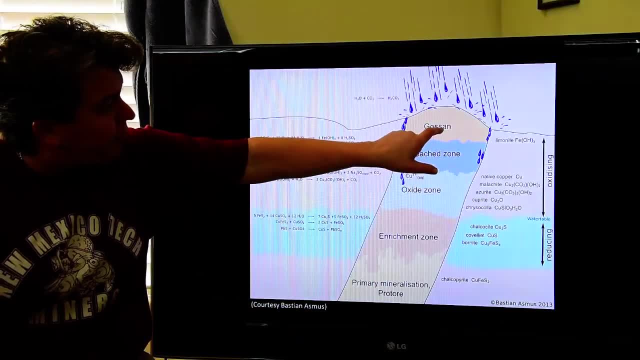 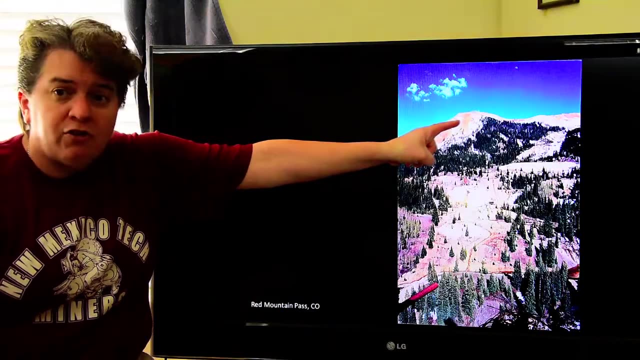 And we see this in. this is Red Mountain Mining District in Colorado. Let me just go back one moment. This thing called the gosson. that's usually a reddish color And so Red Mountain. notice the reddish color up there. 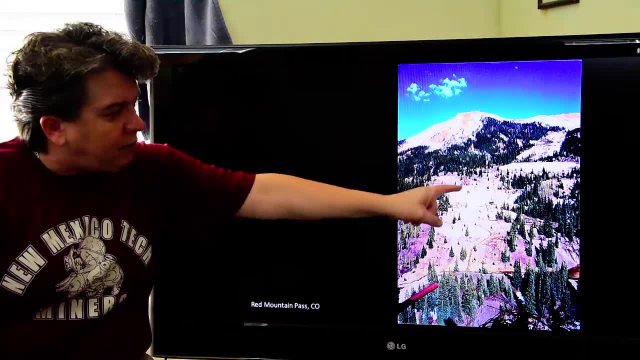 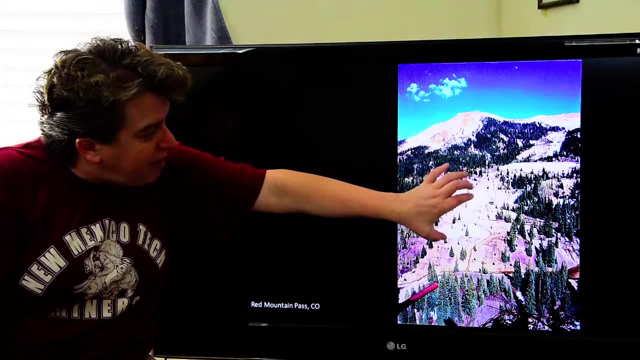 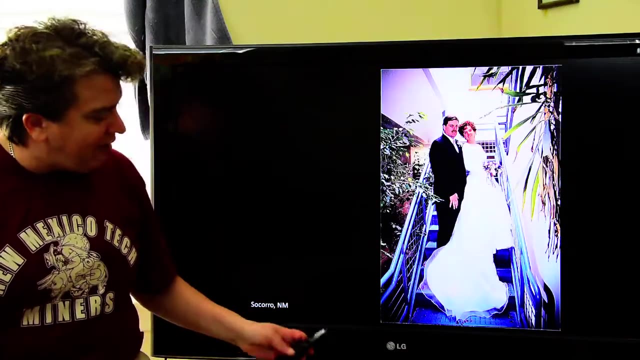 That's the gosson right. So we would imagine the enriched zone should be somewhere down here. And guess what? All of our mines are sitting down here because they were going after that enriched zone of ore. And that brings me to the random picture of the day. 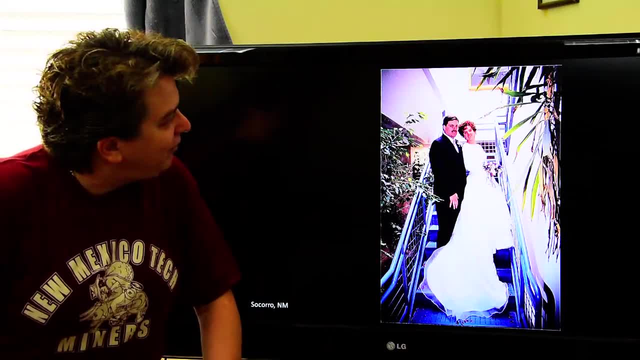 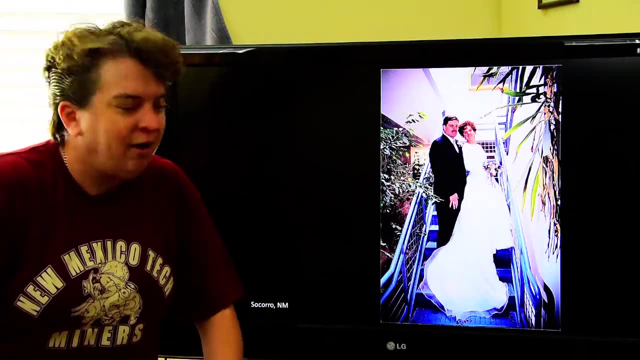 And that's my wedding picture. I like the fact that I'm standing a step above my husband, but I'm still shorter than him, And I wore a dress because you know, hey, it was important that day. I'll wear a dress if it's an important enough day. 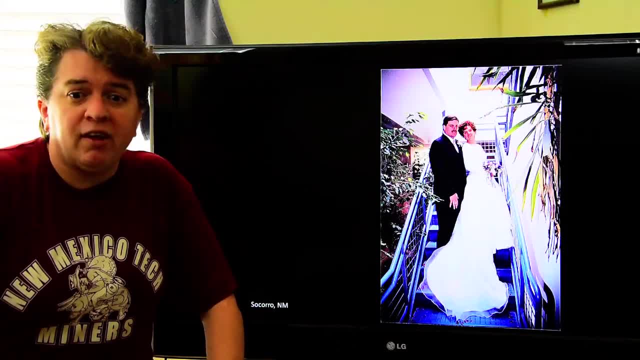 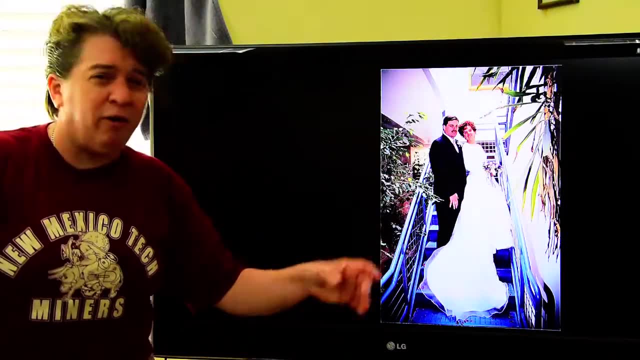 And I'm not going to say any kind of like stupid things, like that was the happiest day of my life. The only day you're allowed to say that is on your wedding day, Because if I said, oh, that was the happiest day of my life was my wedding day. 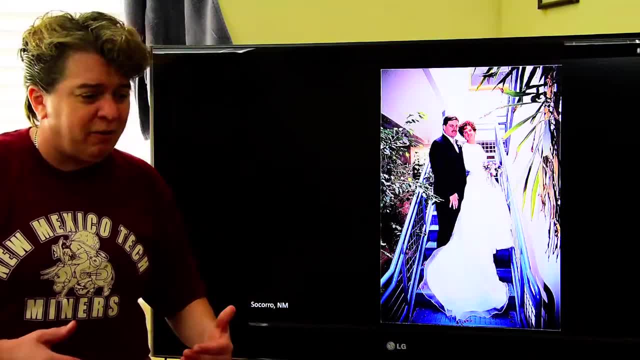 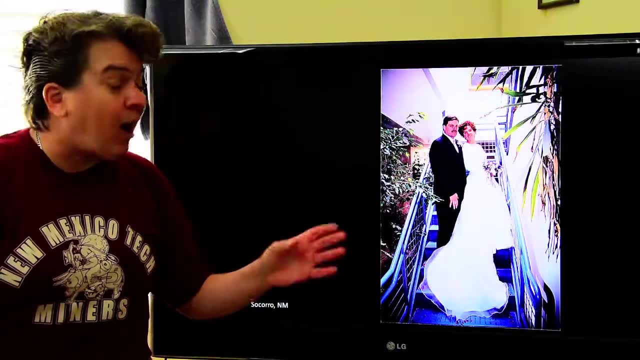 I'm doing something wrong in my marriage because you know that would just be sad, Like it was great the first day and just never was good the day after that. So I'm going to say that was a great day, and every day with my husband. 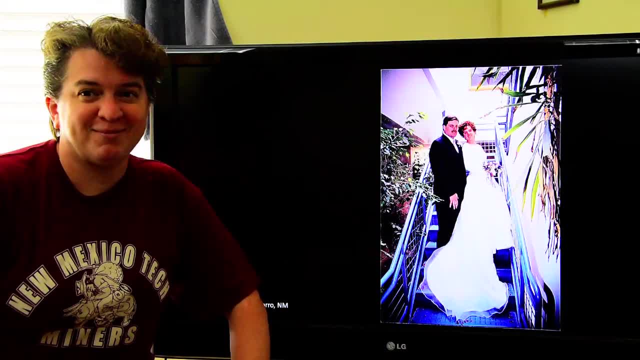 is better than the last Aww. 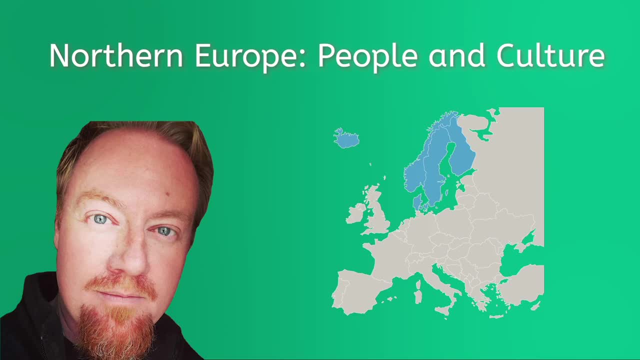 Welcome back, folks, Brian. here and today we continue our tour through Northern Europe and the nations of Denmark, Finland, Sweden, Norway and Iceland. So to begin today's lesson, I'm going to ask you a difficult question related to today's lesson objectives. 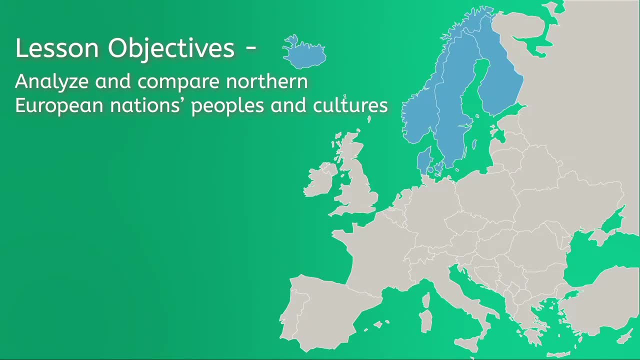 Today we are going to take a comprehensive look at the peoples and cultures of Northern Europe, including population and statistics, ethnicity, religion, language and political and economic structures. So are you ready for that question? Here goes: What do the flags of the nations of Northern Europe all have in common? 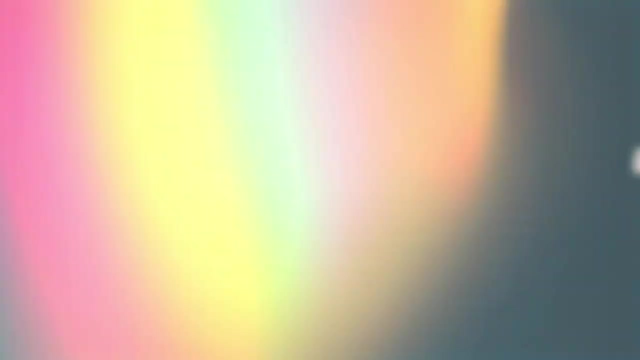 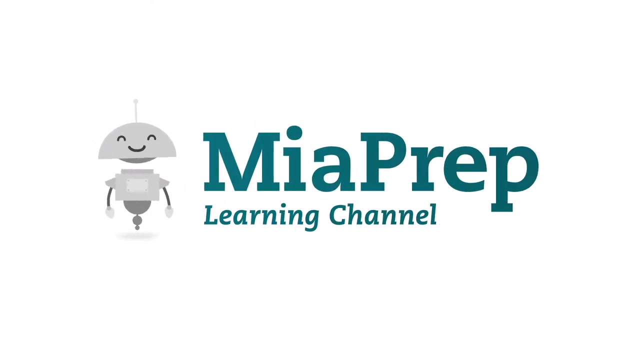 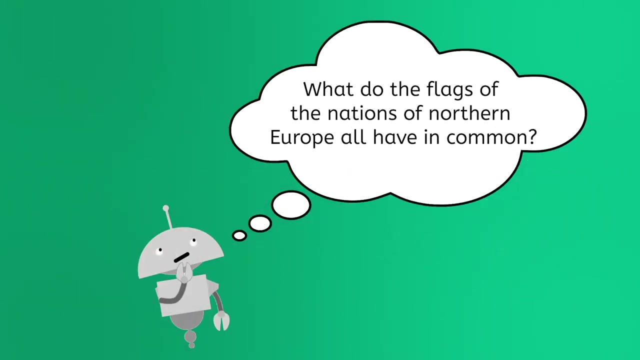 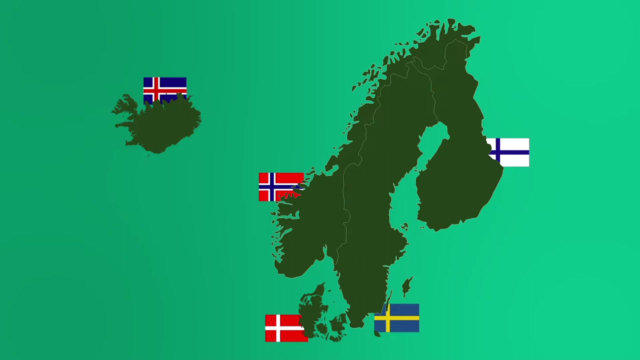 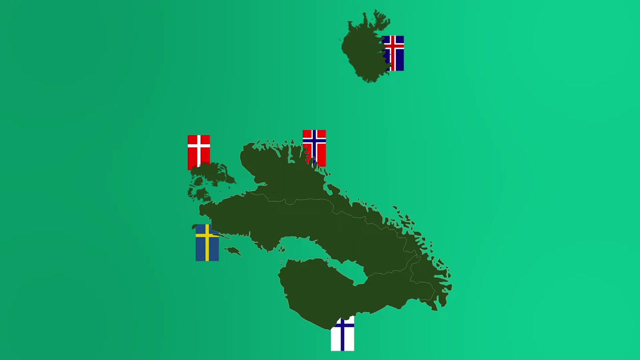 The answer in just a moment. So how'd you do on that question? Ah, come on, it was really easy. If I show you the flags for each country… And what if we do this? Now you see it: The cross embedded into each nation's flag, which tells you a lot about their religious affiliation. 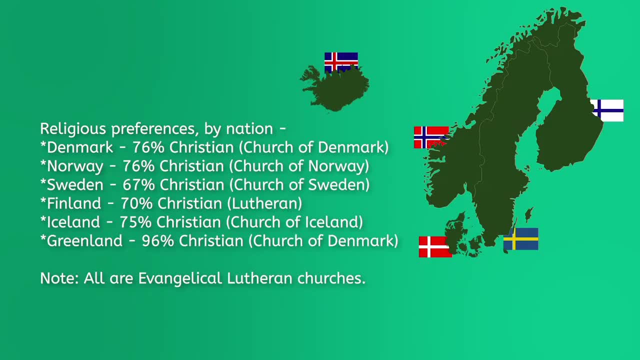 Although the peoples of each nation are predominantly Christian- at least 67% each country's inhabitants- are also largely followers of a geographically specific church, as you can see here. For example, most people in Denmark attend the Church of Denmark. These state-centric denominations…. 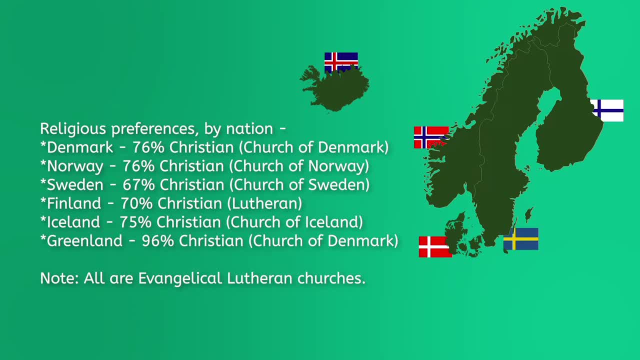 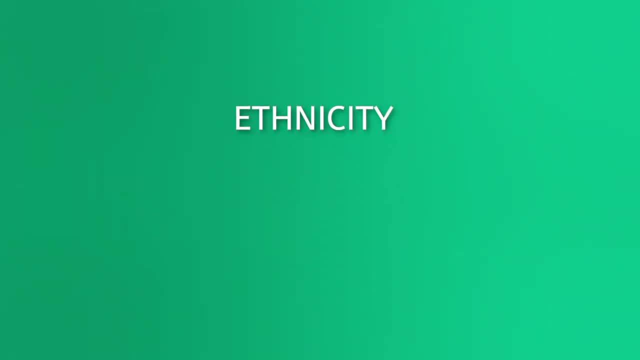 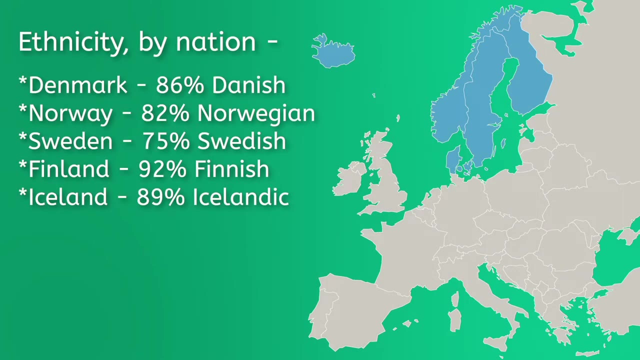 …are similar in that all are like those in Finland: Evangelical Lutheran Churches, which are Protestant religions based on the teachings of Martin Luther. Ethnicity- The ethnic composition of each nation is also largely central to that country, Although the peoples of each nation identify their ethnicity with their home country. all but one are of Northern Germanic heritage, and that would be the Finnish, who are of Baltic ancestry.